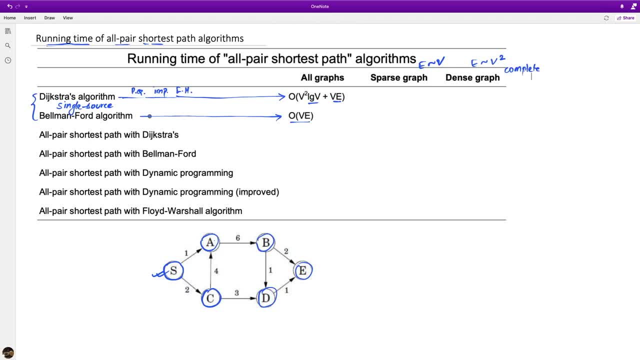 graph. So let's see how these two algorithms' time complexity changes for a sparse graph and dense graph. in a sparse graph, since E is almost close to V, so this becomes big O of V square log V plus V square. and now, since V square log V is bigger than V square I. 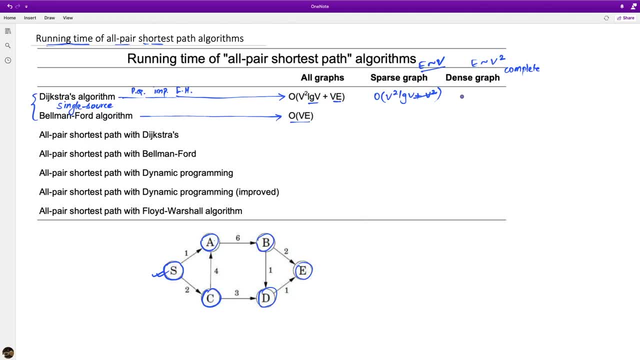 can remove this term, so the running time becomes V square log V. in the case of Danes graph we have E almost close to V square, so this becomes big O of V square log V plus V cube, and since V cube is very high compared to this one, 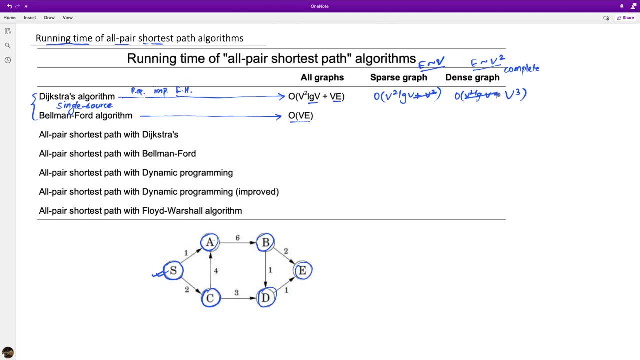 this term goes out, so the running time becomes big O of V cube. similarly for the Bellman-Ford algorithm, since here, in a sparse graph, V is almost equals to E, so the running time becomes big O of V square. and in the case of Danes, graph. 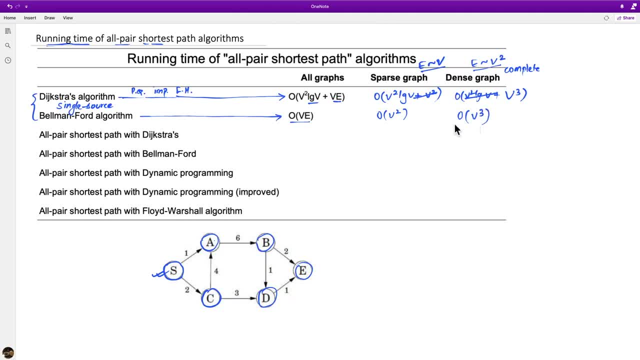 this becomes big O of V cube. one very easy trick to Compute all-pair. shortest path is to simply run one of these two algorithms at every vertex of the graph. so I can run Dijkstra's algorithm with S as my starting vertex and then a as my starting vertex and B as my starting vertex. 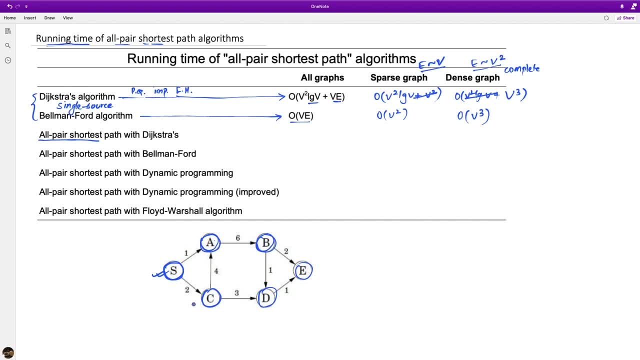 Repeatedly for each of the vertex in my graph and then obtain all-pair shortest path. So if we simply do that, say for example using Dijkstra's algorithm, then the running time of the all-pair shortest path algorithm, the time complexity becomes. so this will be: 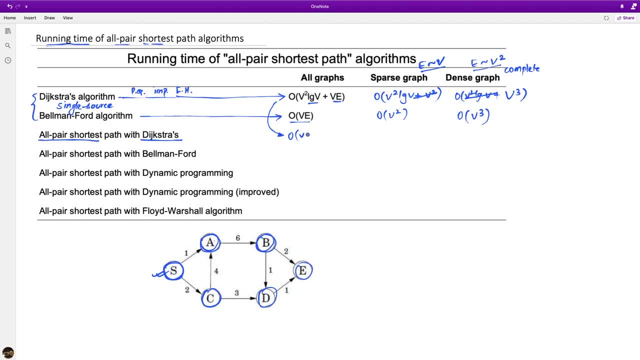 This run V times big O of v times V squared log V plus V. now, in the case of a sparse graph, so this becomes big O of v cubed Log V. and In the case of a dense graph, this becomes big O O of V to the power 4, because V cube run V times becomes V to the power 4.. Similarly, 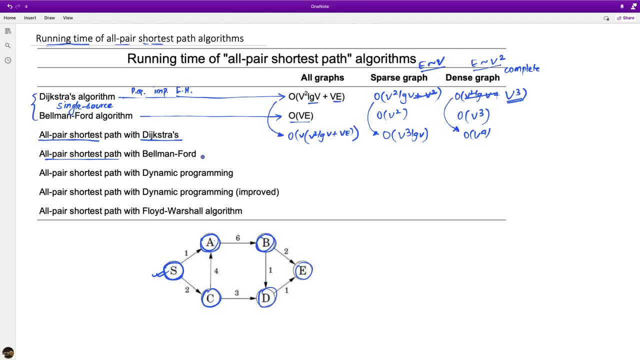 if we want to obtain all pair shortest path with Bellman-Ford algorithm, then the running time here becomes O of V- square E, and in the case of sparse graph this becomes O of V- cube, and in the case of dense graph this becomes O of V to the power 4.. Now, obviously so this. 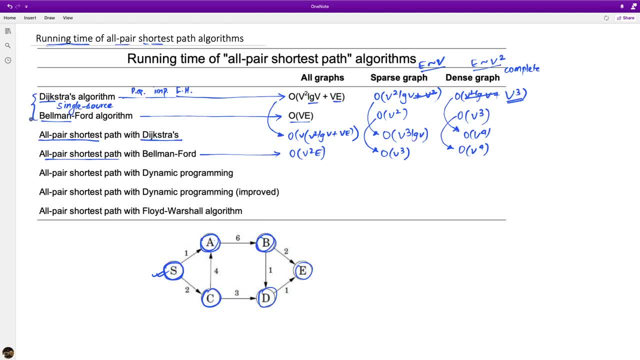 is easy because if I have implemented Akishtra's algorithm or Bellman-Ford algorithm, I can simply obtain all pair shortest paths in my graph by running either of them V times. The question is: can we obtain an algorithm that runs faster than this? that is in the worst. 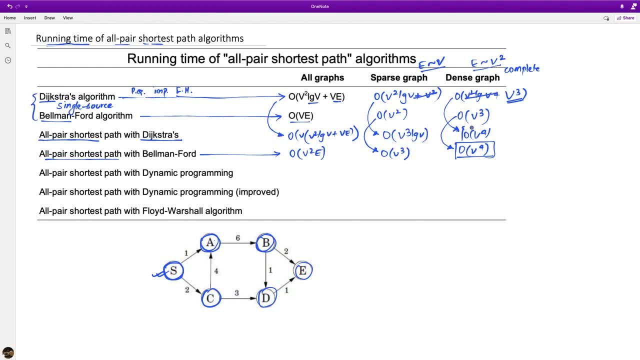 case, this running time is O of V to the power 4, to the power 4.. So can we have an algorithm that can do better than that? So one proposed algorithm is to use dynamic programming to solve the all pair shortest path algorithm. Now the default dynamic programming algorithm: 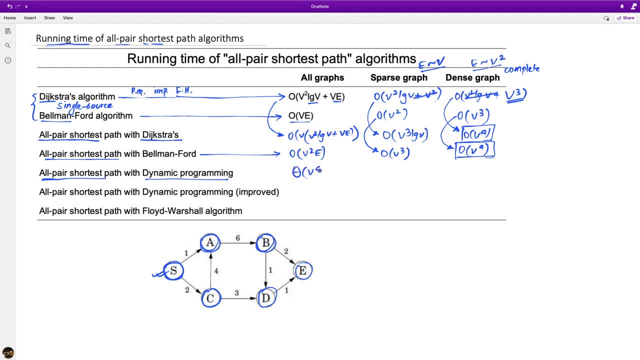 runs in big theta of V to the power 4.. So since this is big theta, whether it is sparse graph or dense graph, the running time stays the same. So this isn't very exciting, because this is same as the time that it would need if we called Bellman-Ford or Akishtra's. 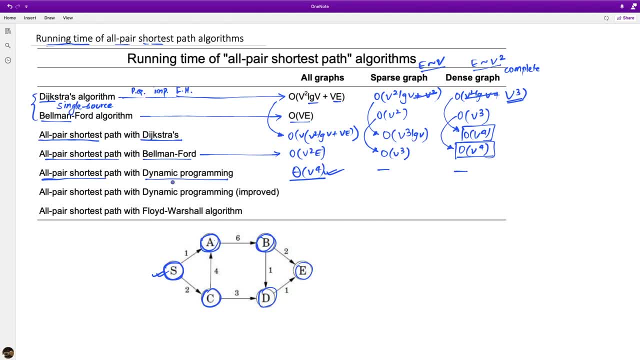 V times, But then with some improvements to this dynamic programming algorithm. if we improve the algorithm, this can actually run in big theta of V cube log V time, which is improvement. And since this is big theta, whether the graph is sparse or dense, that will also. 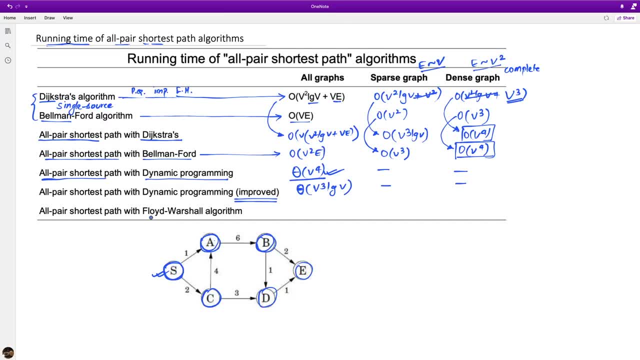 always be the running time. Now, however, the Floyd-Warsall algorithm further improves the time complexity and this gives us big theta of V-cube time complexity. and since this is big theta, whether it is sparse graph or dense graph, the running time becomes the same. So dynamic programming implementation. 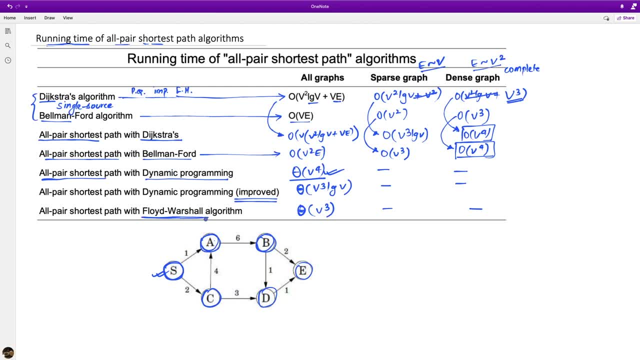 is not faster than the Floyd-Warsall algorithm, but it lays out some foundation that are helpful for us to understand how Floyd-Warsall works. Now, this is dynamic programming. this extends the recursive implementation of the overall algorithm and then use this greedy approach to achieve this running time of big theta v cubed.